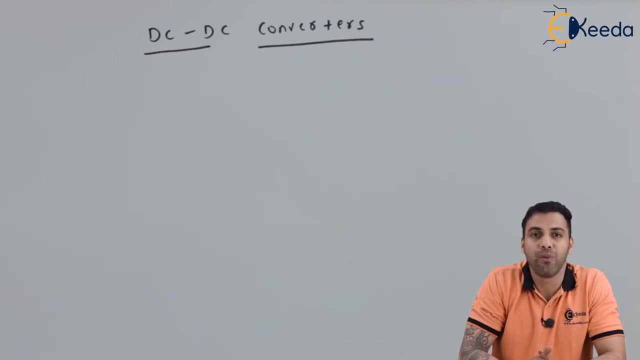 Which we take, for example, MOSFET or IGBT, and we control the switching operation or we control the gate pulse, so that we will be getting an output voltage which is either higher than the input voltage supply, which is DC, or we will be getting a low value of the output DC voltage compared to the input DC voltage. 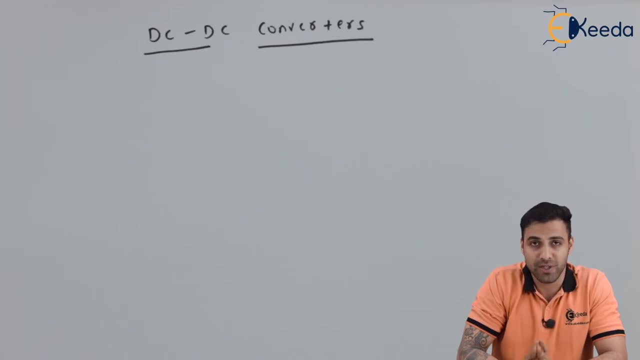 So, friends, as all the DC to DC converters require a switching device, and all the switching device gets controlled, or all the switching devices can be controlled through gate pulse, So we get the output voltages accordingly. First of all, our DC to DC converters are divided into several parts. 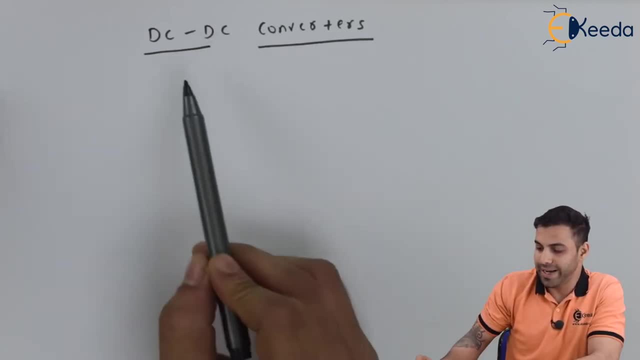 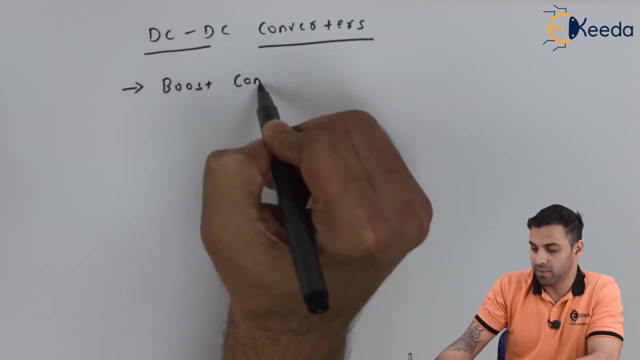 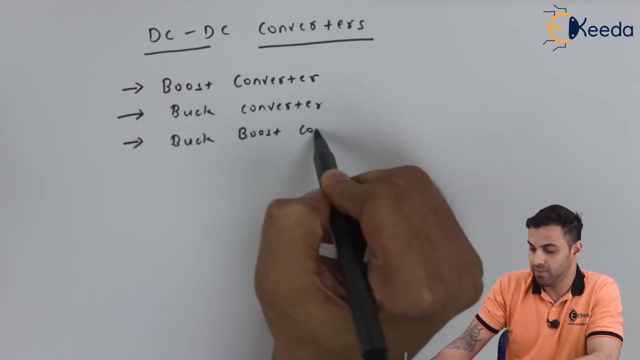 Let's see what those parts are. So, friends, if you can see here, DC to DC converters are divided into number one boost converter, Number two is a buck converter, Number three is buck boost converter And number four would be a cook converter. 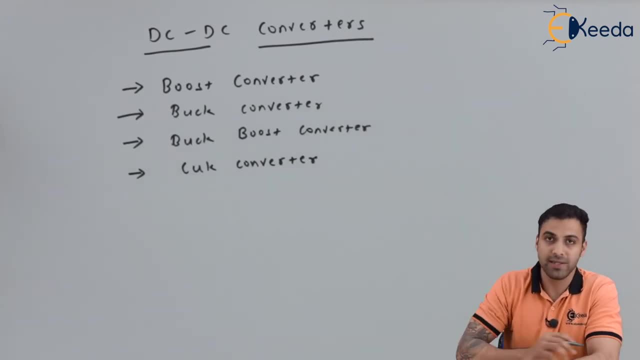 So, friends, boost converter is a device or a power converting device or a switching regulating device that converts a low value of DC voltage to a higher value of DC voltage. That's called a boost converter, which we will be discussing in the upcoming lectures or in detail in this lecture. 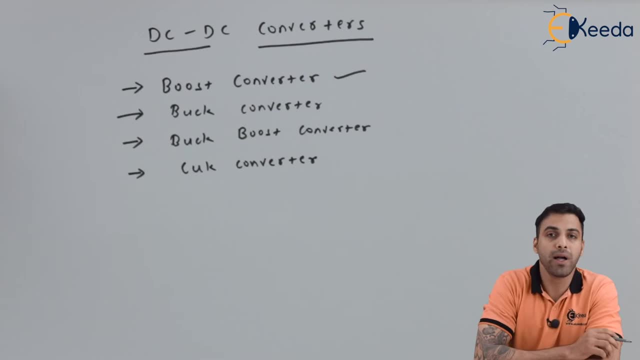 So now let's talk about DC to DC converters. Let's talk about DC to DC converters. So let's talk about a buck converter. So a buck converter is a device which converts a value of DC input to comparatively low value of DC output. 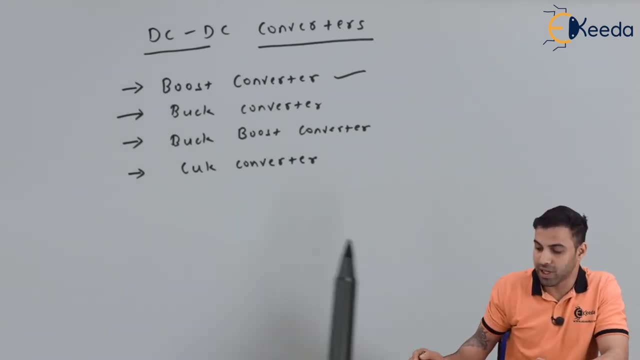 So that's called a buck converter And the buck boost converter. as the name suggests, it can either convert a low value of DC to a high value of DC or a high value of DC to a low value of DC, And the cook converter is a new converter that comes into existence. 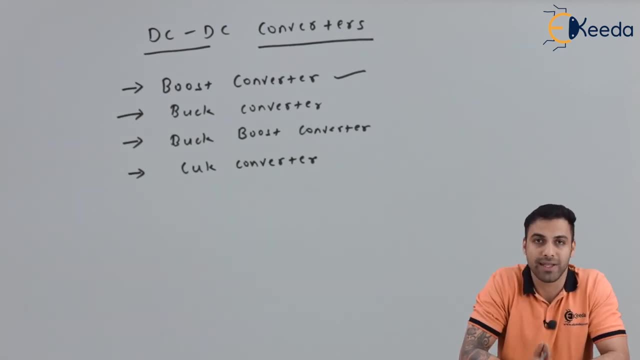 which we will be discussing in detail in the end of this lecture. So, friends, let's start with a converter which converts a high value of DC input to comparatively low value of DC output. That is called a buck converter. So, friends, to operate any of these converters.